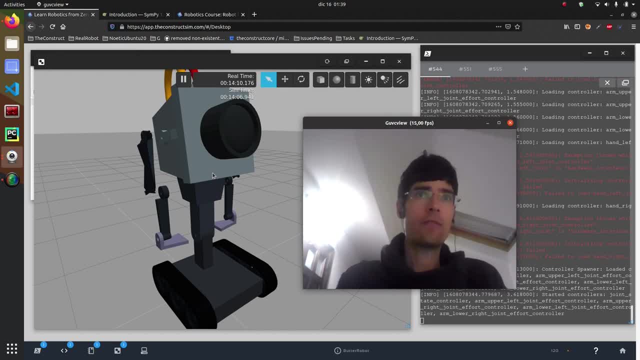 why do you need it? Because if you want to do this kind of applications, if you want to do robots that walk, robots that run, robots that manipulate stuff in an intelligent way, it's the way to go, And also if you want to practice some math, it's also a very good place to start. So here, what we are going to do is a very simple example, which is calculating the. 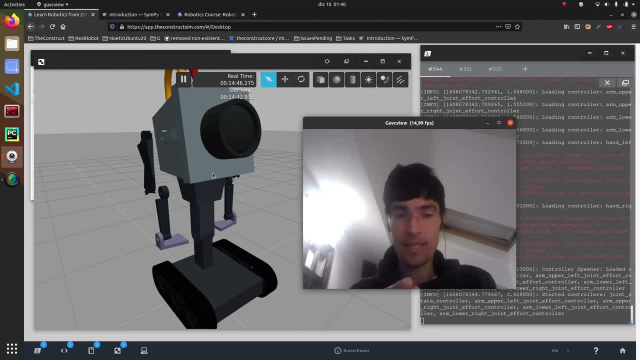 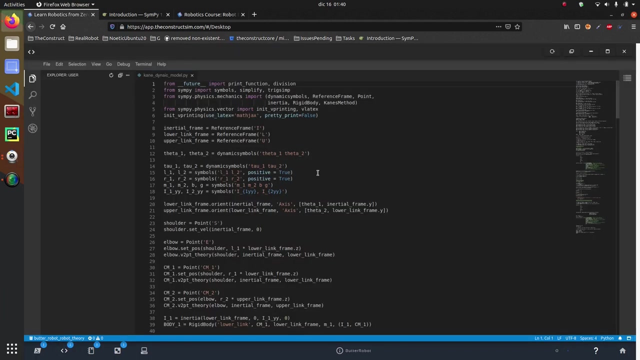 dynamic model of the robot, of the, in this case the robot arms, And through that we're going to make it maintain a position, or try to maintain the position. Okay, so let me show you, through the code, a bit how this is made. So, essentially, what we're doing is solving a differential model of the robot. 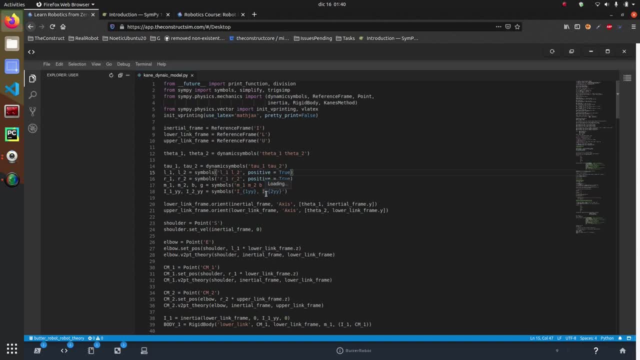 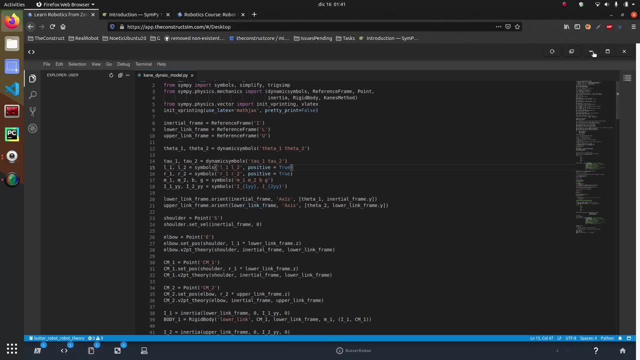 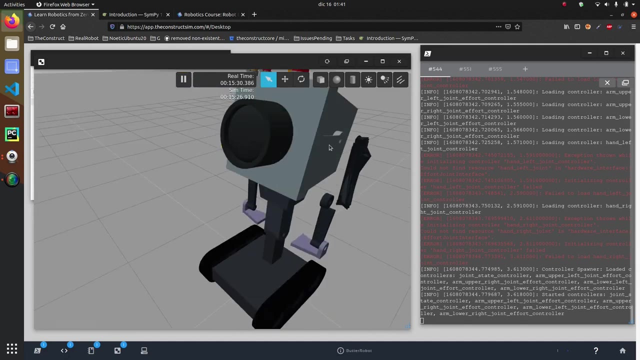 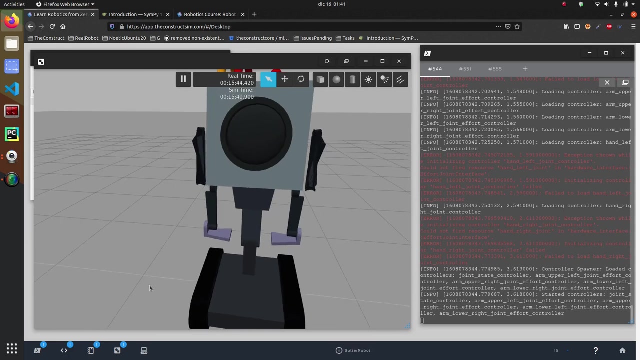 equation, which is a model that is based on various assumptions, but the most important assumption is that we're only moving in a plane, so the arms here will only move in the y-axis, let's say they only will rotate there and they won't move out outwards. that's a very big assumption, but from for the 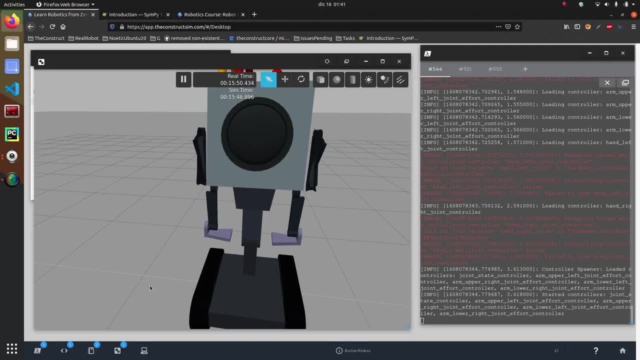 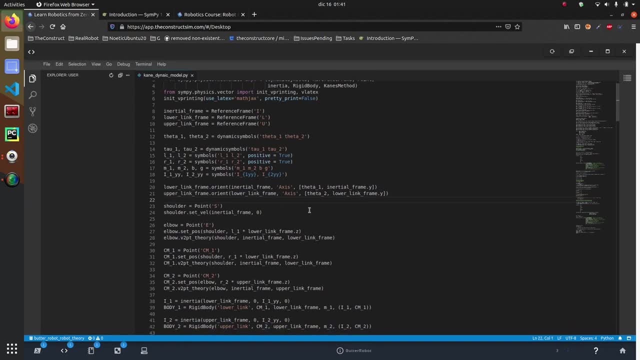 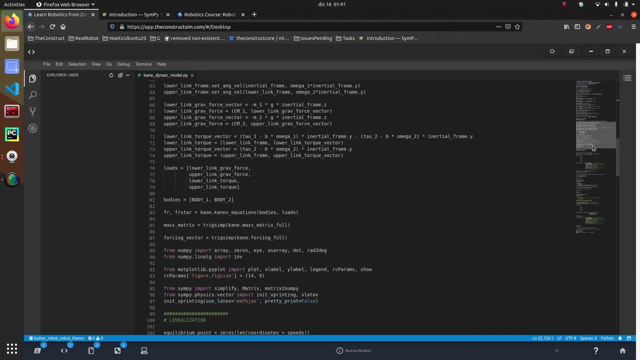 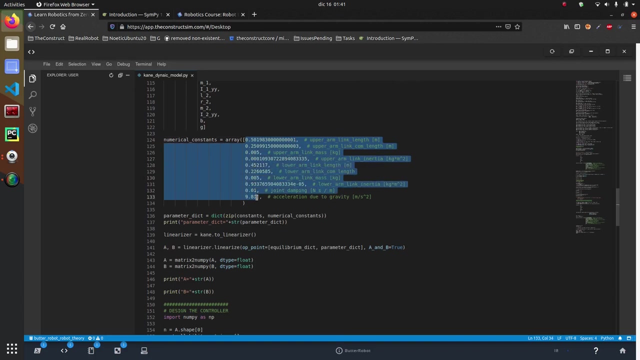 start. I think it's more than enough, because this is a very deep topic and also it's quite complex in the mathematical terms. so essentially, what we do is we create a model and we solve a differential equation. and once we have a model, based on its impact and the 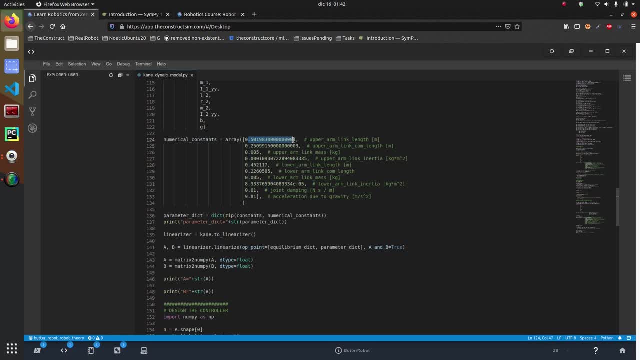 architecture that we're using for the model. then we kind of solve a differential question as such, based on the parameters of our robot arm, in this case, which is a two link system with the length of the arm, the position of the center of mass, of the of the first link and then the mass. 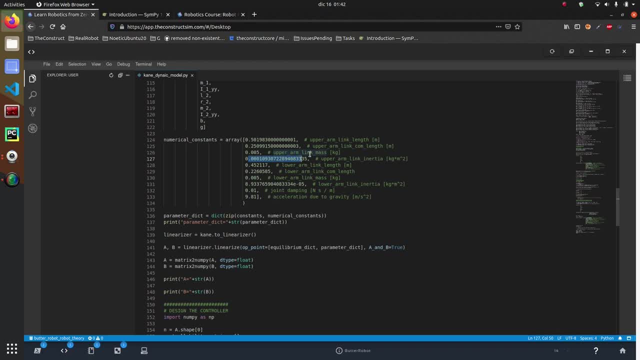 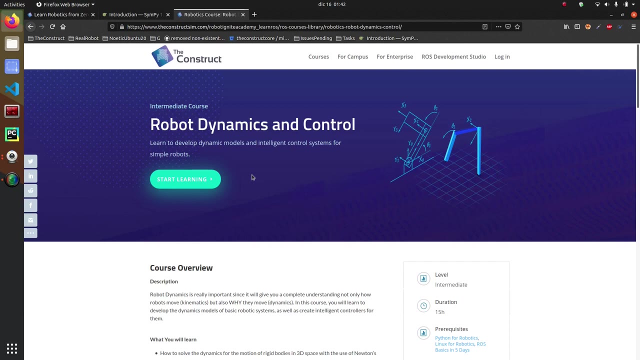 We can calculate the inertia through various methods and everything that I'm explaining here. it's explained much in detail in this course on robot dynamics and control. So if you're interested in this, have a look at this course, because it helped me a lot to get started, at least in this very tiny, tiny demo. 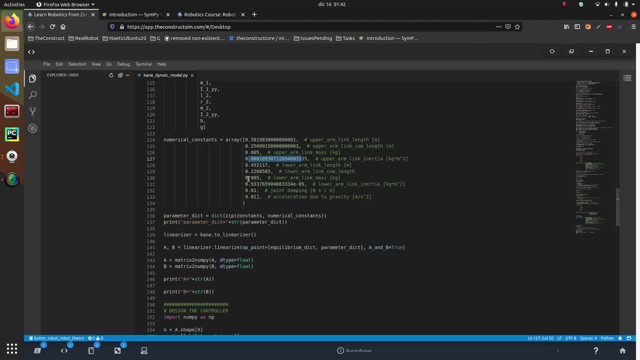 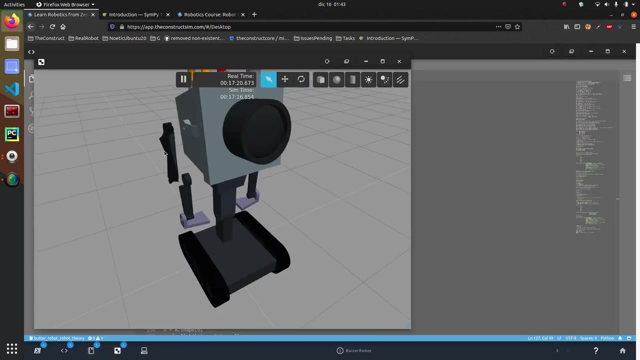 Yeah, and so here we calculate this inertia for the arm, the part, this part here. let me show you this part here, this one. and then we do the same thing with the lower part, which would be the one here. 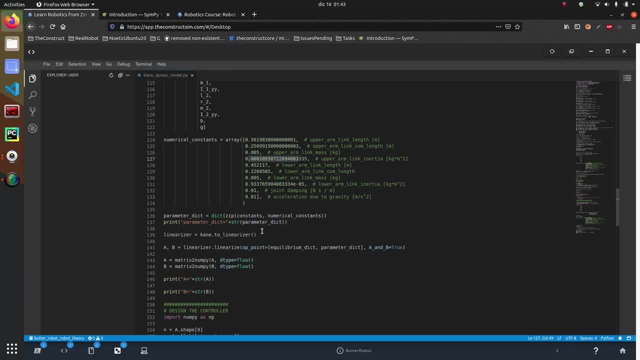 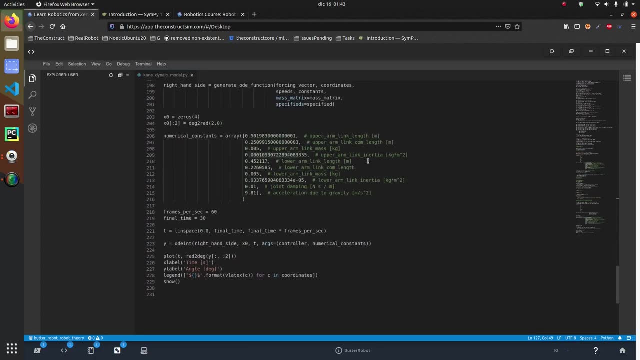 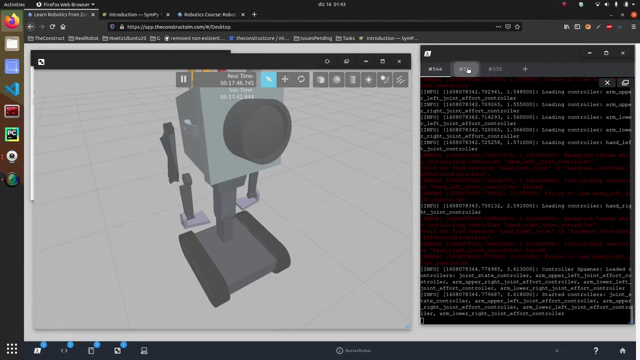 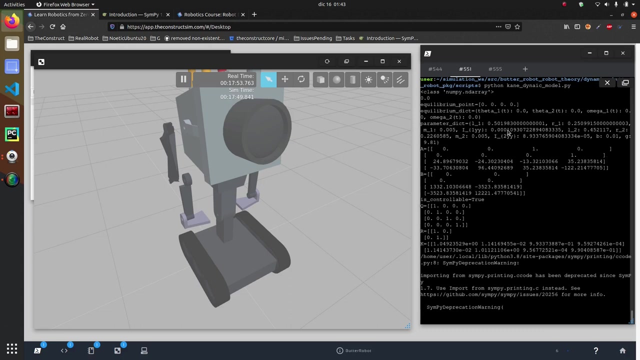 Yeah, and once we have it, then it's, It calculates the parameters and essentially it solves and gives us a matrix. So let me just show you: There we go, So there you go. So at the end what we have is we specify the point of equilibrium. 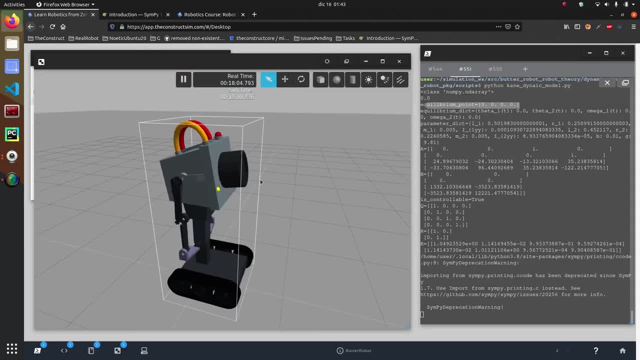 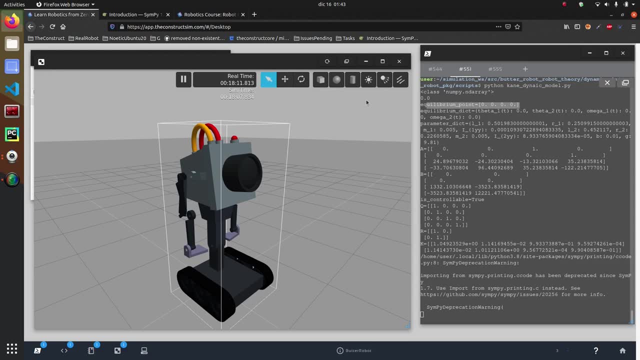 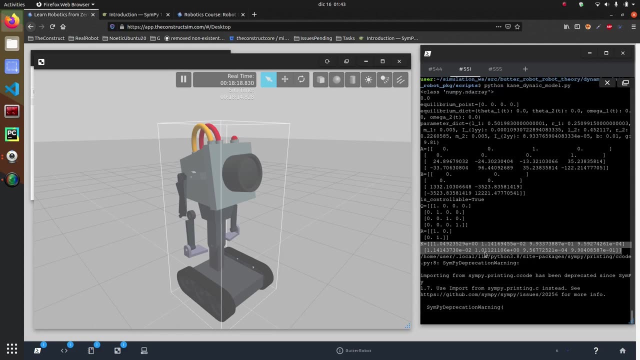 So the point in which we want, We want to maintain the arms, So in this case, zero, zero, which is the arms upwards, And then, after calculating and solving the differential equation, we have these parameters that we will use to do a very basic, very crude linear controller through dynamics. 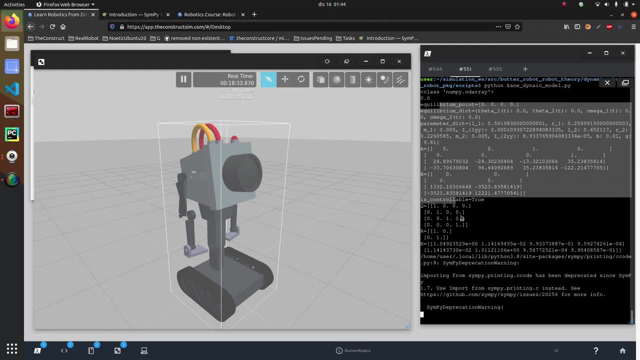 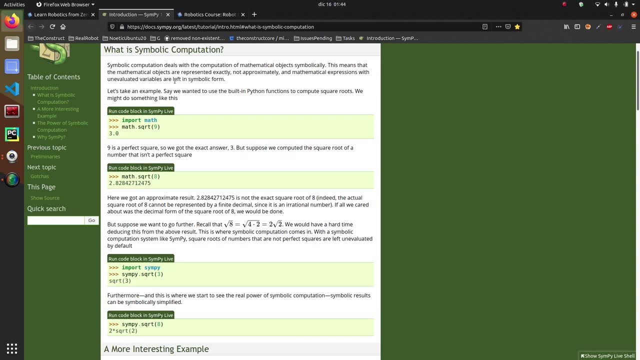 Yeah, Yeah. So the thing that you see here, all the calculations, most of it it's used through symbolic computation in Python. If you want to know more, I'll leave in the video description a link to this page which gives you a very good tutorial on how to use it. 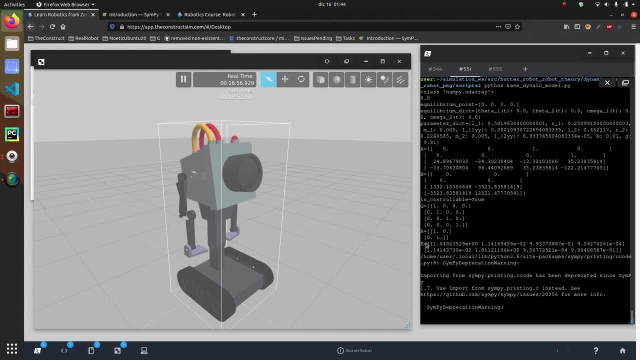 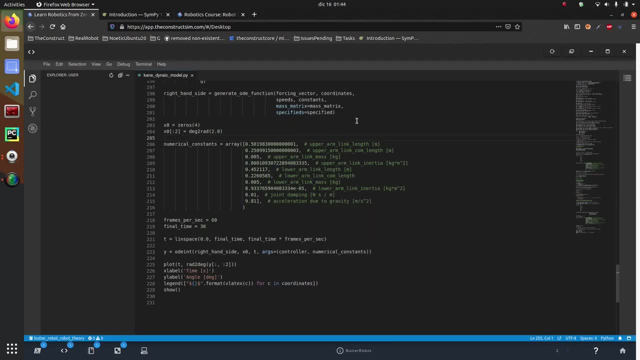 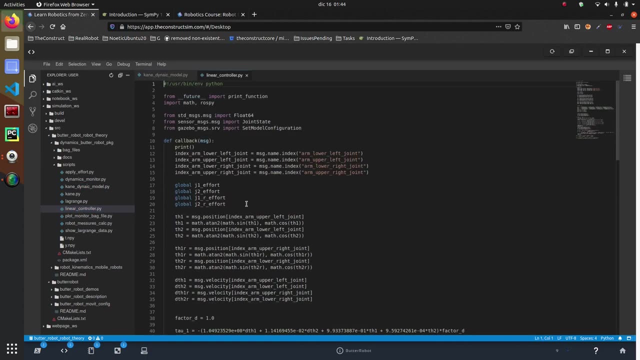 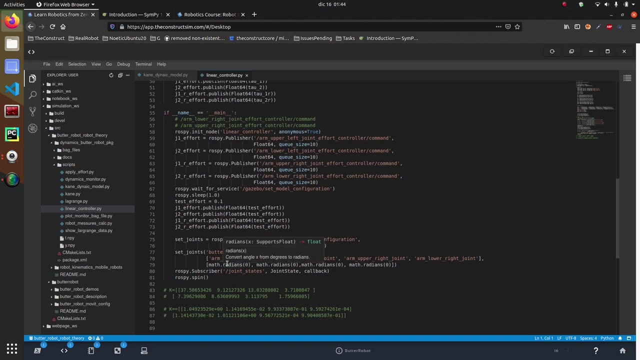 Yeah, So once we have these values, we then put it in our linear controller. Yeah, So let me have a look here to my linear controller. There we go. So my linear controller will use those parameters that I've calculated through the differential equation solution. 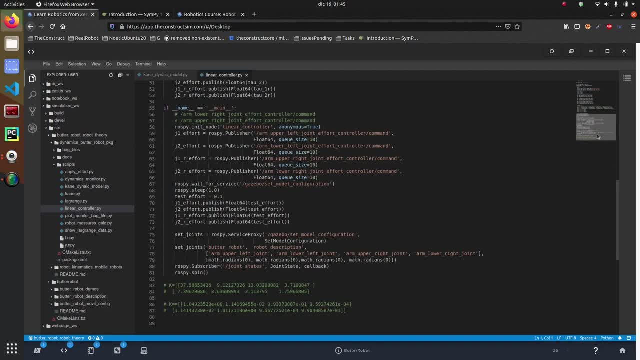 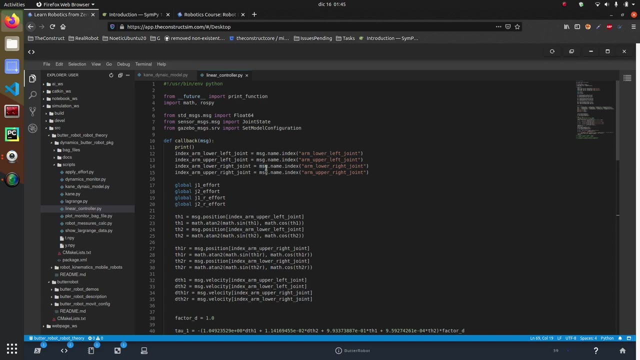 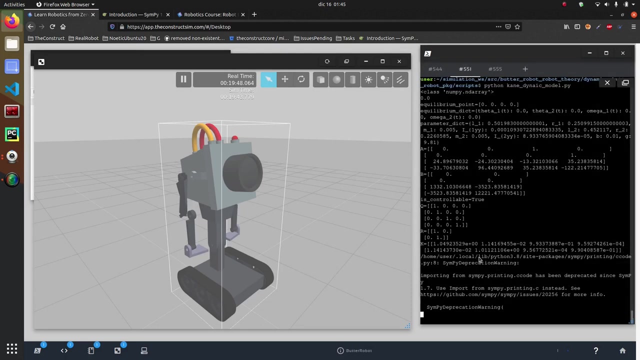 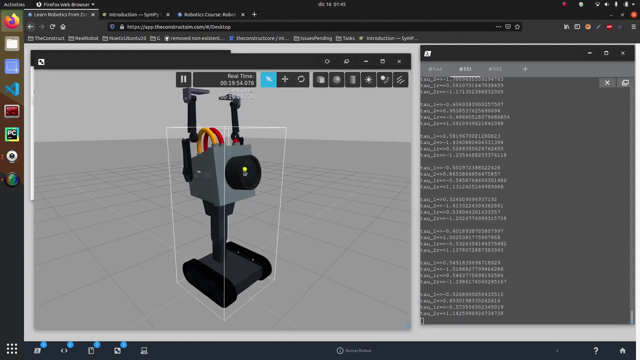 And what I'll do here is I'll give it a very tiny effort And then it will try to maintain the position of equilibrium. Okay, So let me just show you, And there you go. So, as you can see, it's not perfect for various reasons. 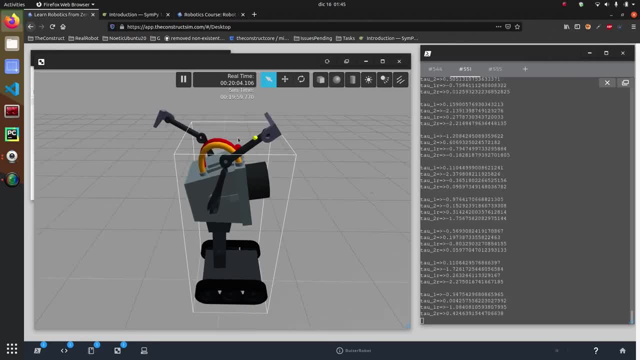 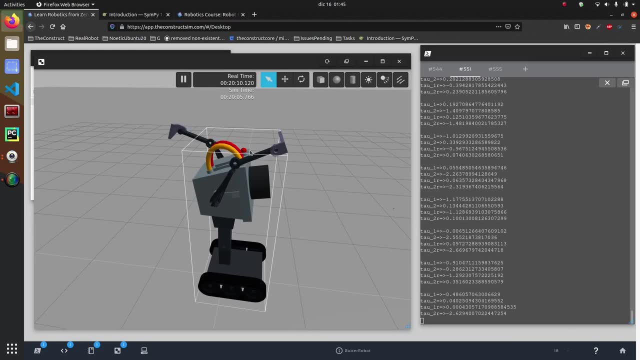 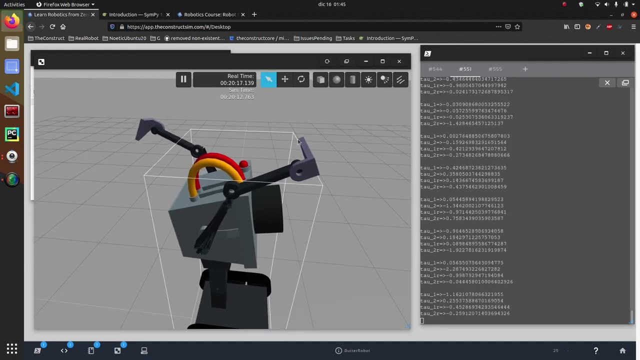 Mainly because I didn't put the exact amount of all of the positions of the inertias And also because the model I'm adding here a mass that it's not included in the model, So it could change the dynamics, of course. 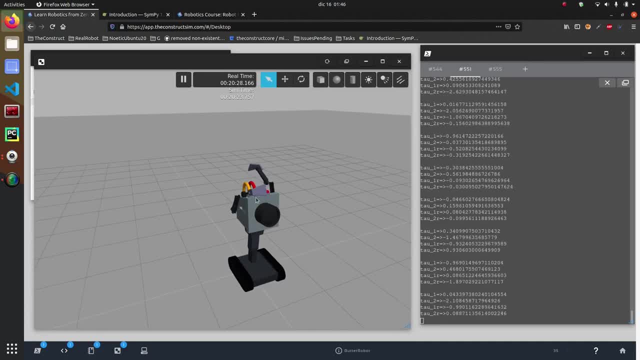 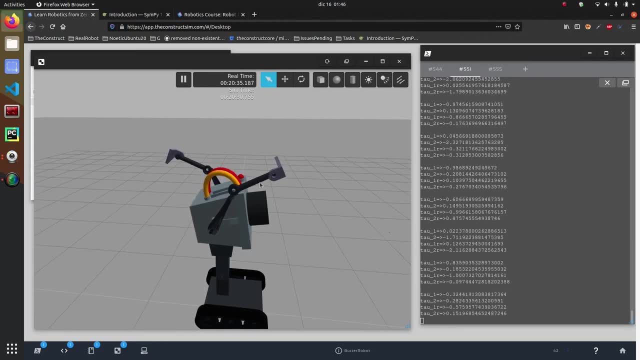 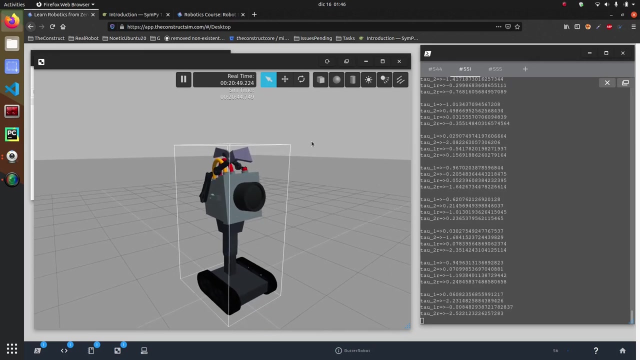 But with a bit of tuning you could get it to work quite well. Yeah, And taking into account that this is controlling itself only through dynamics, Through a model and through a dynamics. So it's quite interesting, quite cool, And that's it for today. 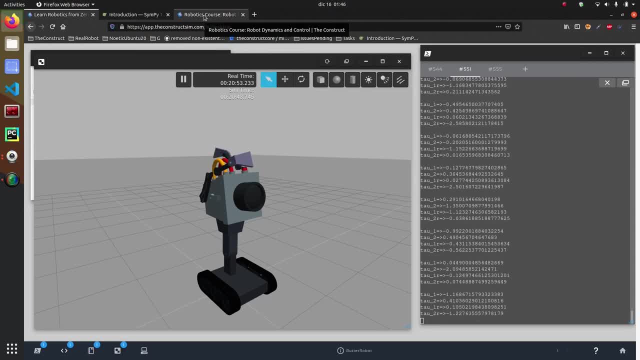 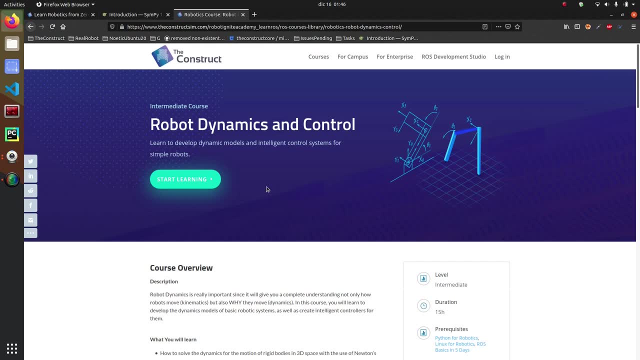 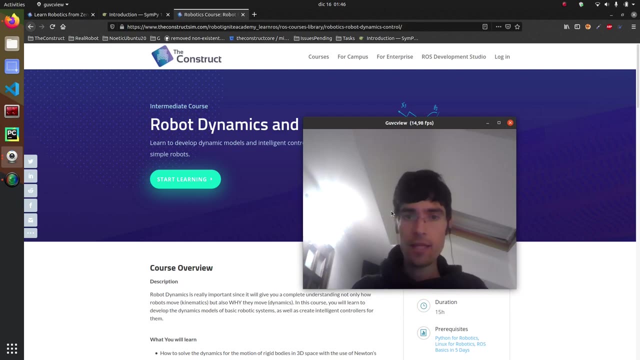 So if you want to know the details, all the steps and extra exercises and how to calculate trajectories, everything you can go to this course on Robot Dynamics and Control. And yeah, that's all for today. So thanks a lot for seeing the video. And see you in the next video. Bye.